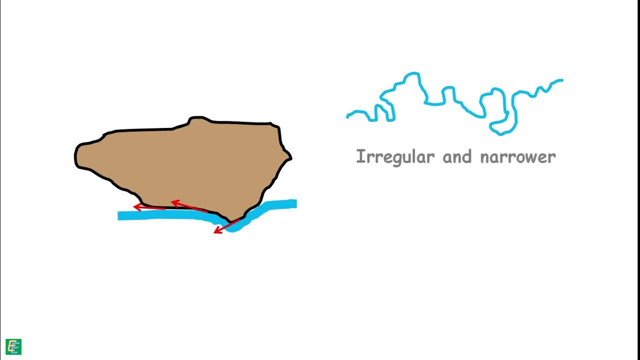 is the resistance posed to the water flowing. While more open the voids, greater is the ease with which the water flows. which water flows through the soil? This property of the soil which permits the water or any liquid to flow through its voids. 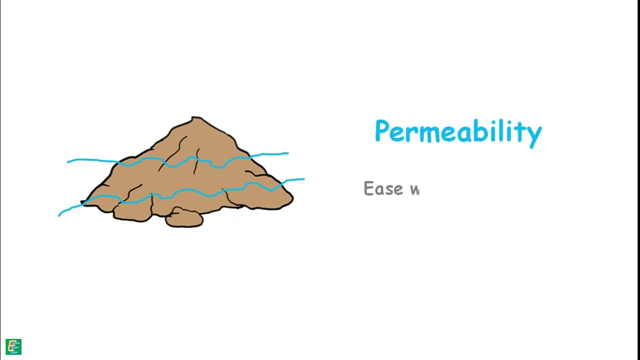 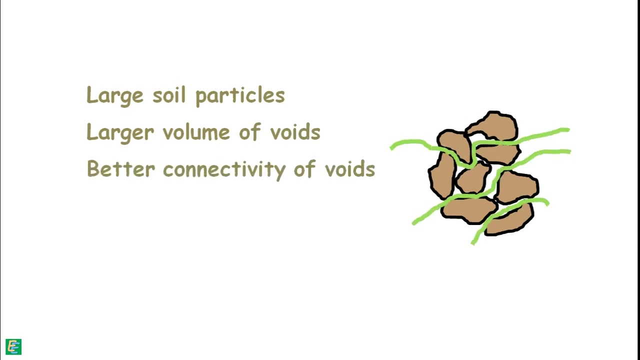 is called permeability. It is the ease with which water can flow through the soil. Gravel particles are large. Larger the soil grains, larger will be the volume of voids and better will be the connectivity of those pores. Consequently, large amount of water may flow through them easily and higher will be the 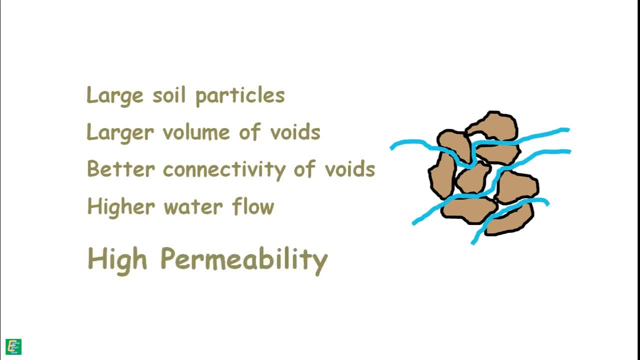 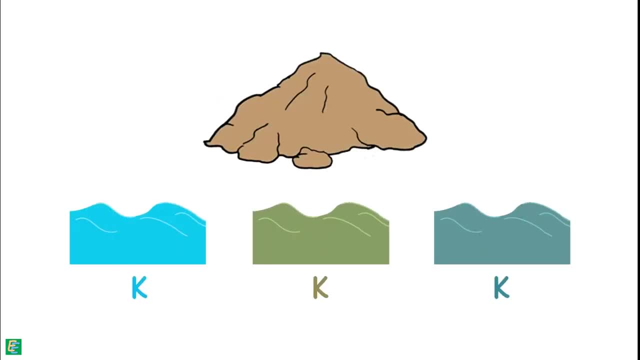 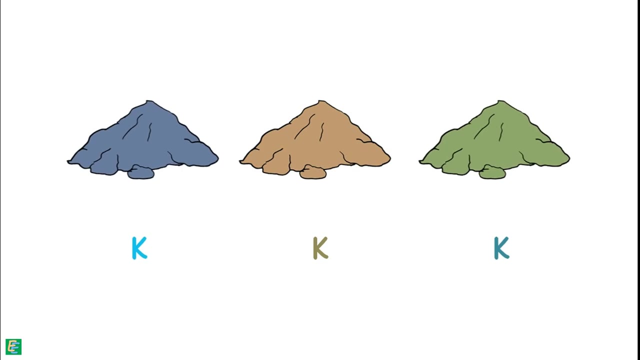 flow of water and that we say higher is the permeability of soil. A soil has different values of permeability for the different liquids, but we will focus only on soils permeability with water. There is a huge difference in the permeability of different soils. 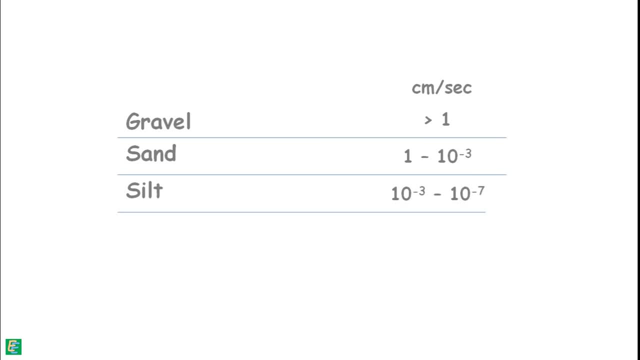 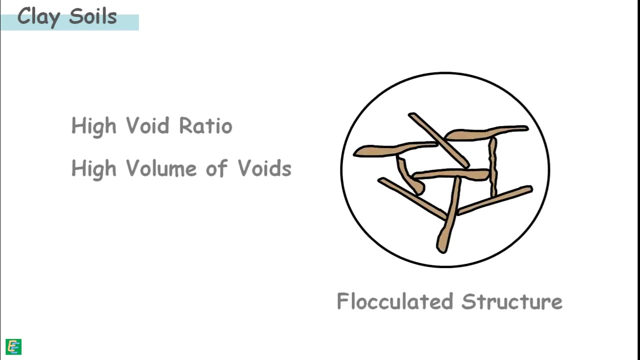 These are the values of permeability of different soils. Gravel soils are most permeable, while clay soils are least. Clay soils have high void ratio as they have large volume of voids because of their flocculated structure. These voids look very large, but it is much zoomed view and because the clay particles 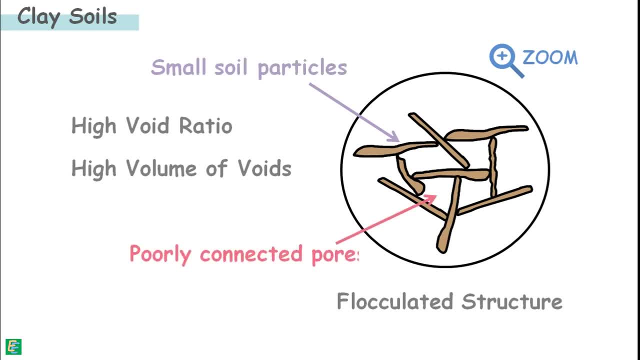 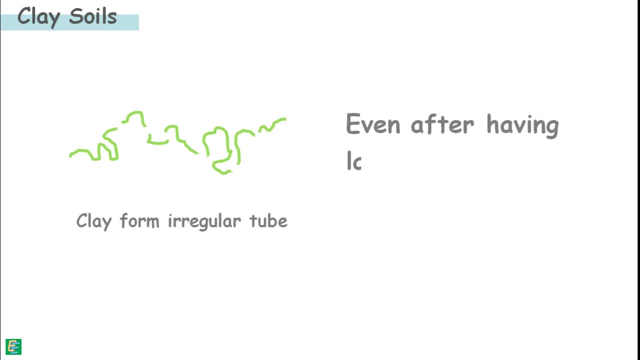 are being very small. these voids are poorly connected to each other and do not form a regular tube or channel like structure. Hence, Even after having large amount of voids, the clay soils are very less permeable. When a soil has extremely low permeability, it is termed as impervious soil. 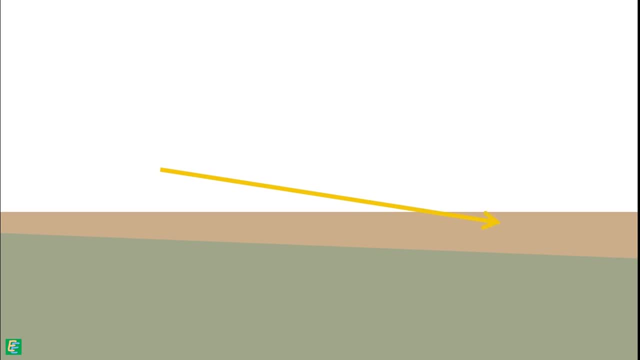 Water in the soil flows from one point to another only if there is a difference of hydraulic head. The hydraulic head is the amount of mechanical energy available at any point in the water. From Bernoulli's principle, the total head or total energy at a given point in the fluid. 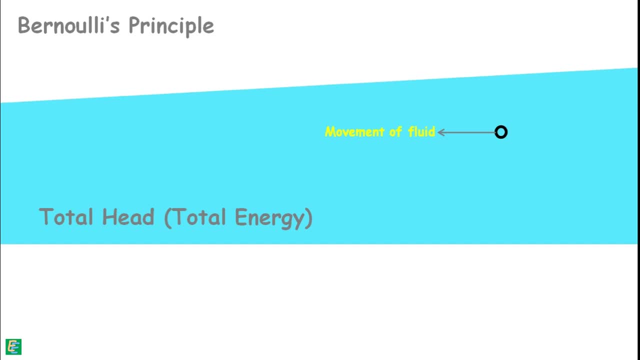 is the energy due to the movement of the fluid, which we call velocity head plus energy. from the pressure in the fluid, which is called pressure head plus energy. from the height of the fluid relative to any arbitrary datum, which is called elevation head. Datum can be understood as any reference line or plane. 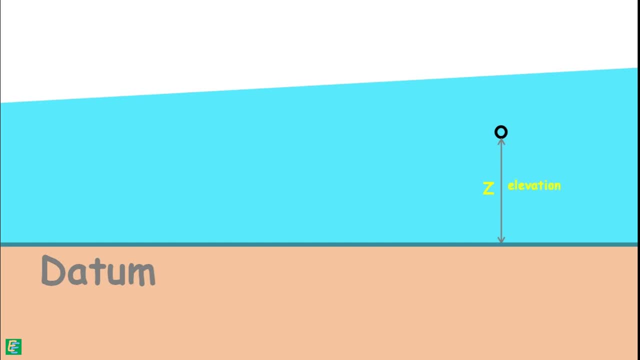 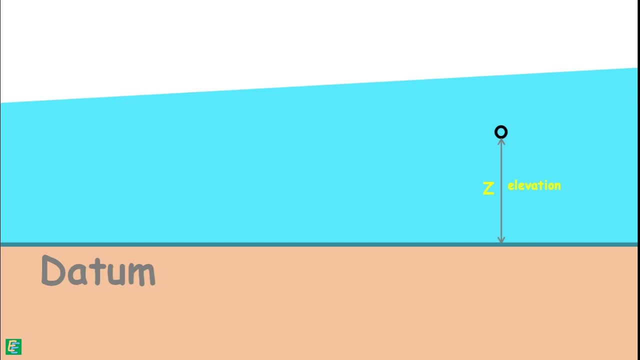 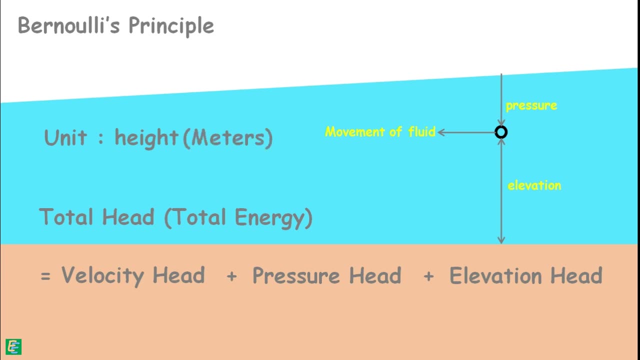 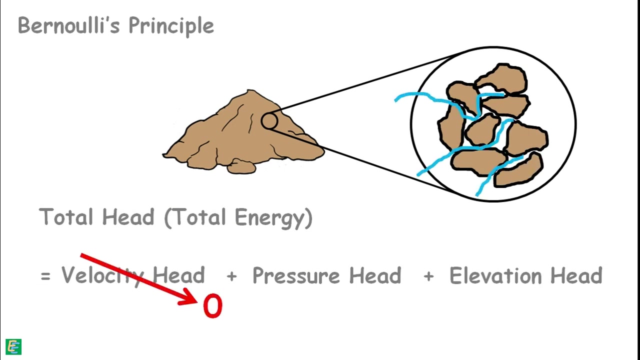 Here z is the reference line. Here a bralette represents the height or elevation of the point of consideration. from our consideration datum, This total head has the unit of height, such as meters. When water flows through the soils, its velocity is very small. Therefore we neglect the velocity head. 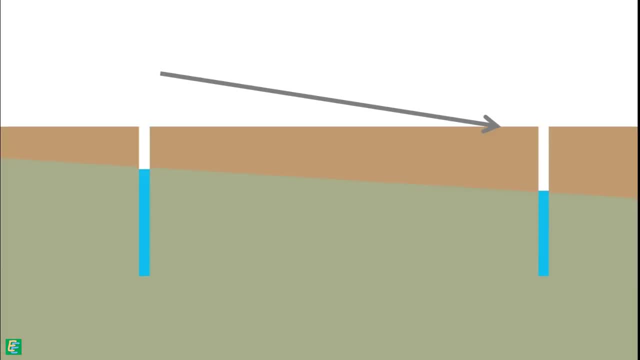 Water flows from high energy region to lower energy region. If hydraulic head of point A is higher than the head of B, water may flow from point A to B. Similarly, if head of B is higher than head of A, water may flow from point B to A. Water does not flow if the point A and B have the 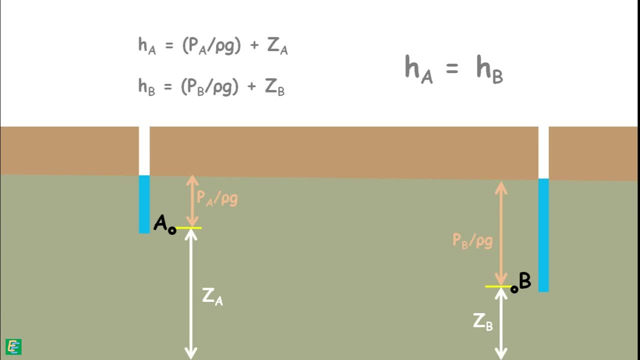 same energy or have inadequate head difference. Because even if A has higher elevation than point B, the hydraulic gradient of both the points is the same. Because hydraulic gradient, which is the sum of both elevation head and pressure head of both the points, is same, Elevation of point A is higher than that of point B. But suppose 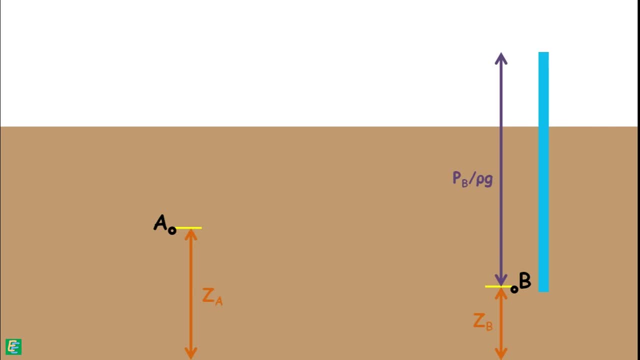 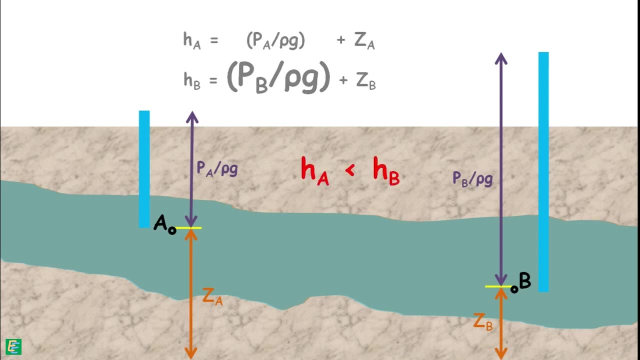 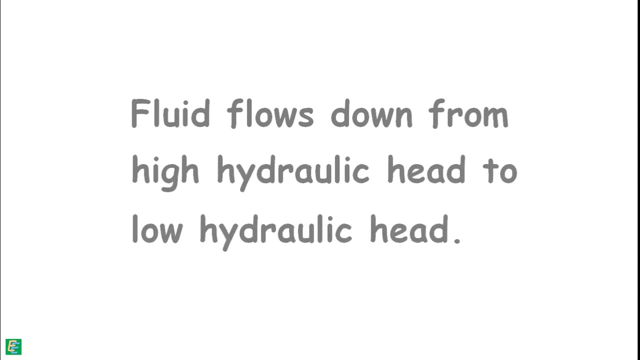 if point B has high pressure head because of any geological confined aquifer conditions, then total head of point B may be higher than that of point A. In that case water will flow from point B to A even against B. Note that fluid flows down from high hydraulic head to low hydraulic head. 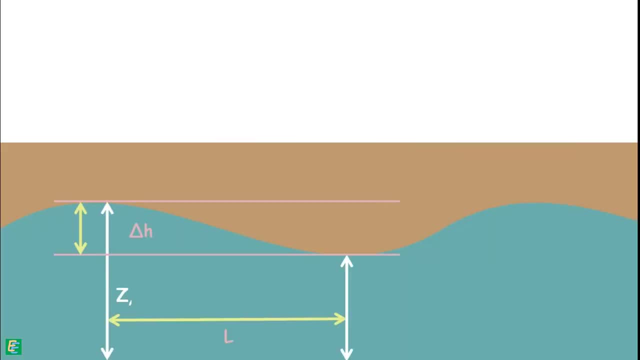 The change in the hydraulic head per unit distance over which this change occurs is called hydraulic gradient. It is written as: this Hydraulic gradient is determined by making several wells at some distances and measuring the water level in them. For example, To measure the hydraulic gradient of ground water, we make two wells in the ground thousand. 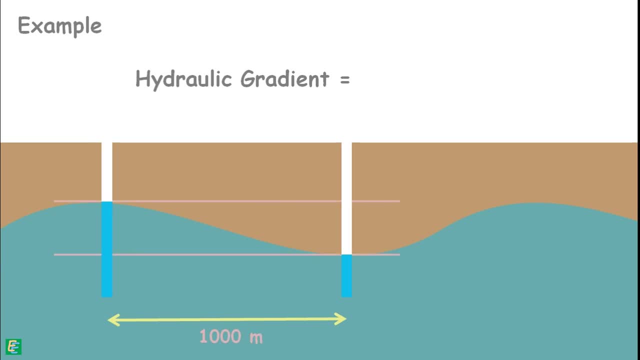 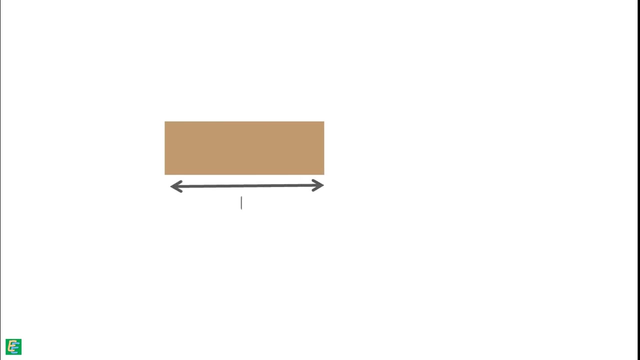 meters apart and measure the difference of water level in them. If the difference of water level in these two wells is 2 meter, the hydraulic gradient is 2 by 1000 or 0.002.. We take a soil sample of length L and, having a cross-sectional area of A, We subject it. 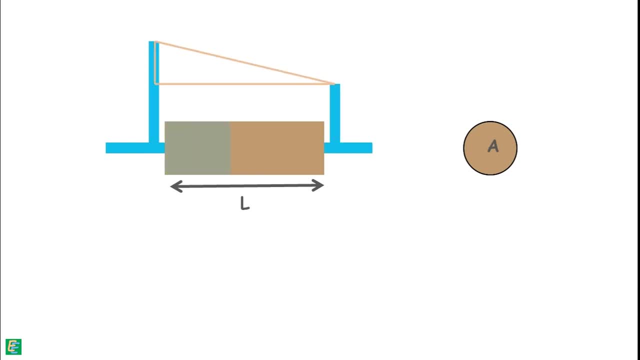 to some hydraulic gradient. We also measure the output discharge of water through this soil. We can get the velocity of flow through the soil by continuity equation, as velocity equal to discharge divided by the cross sectional area of the soil. We increase the hydraulic gradient and for different hydraulic gradient values we note 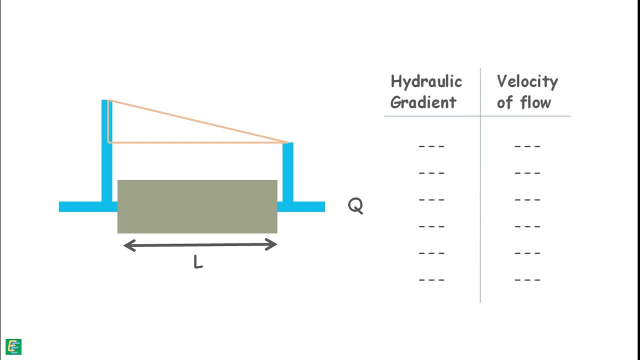 down the corresponding velocity of water through the soil. We plot a graph between these obtained values of hydraulic gradient applied to the external remark. Here we zero the velocity of water nella water by 2m per meter minus the density of water across the soil. 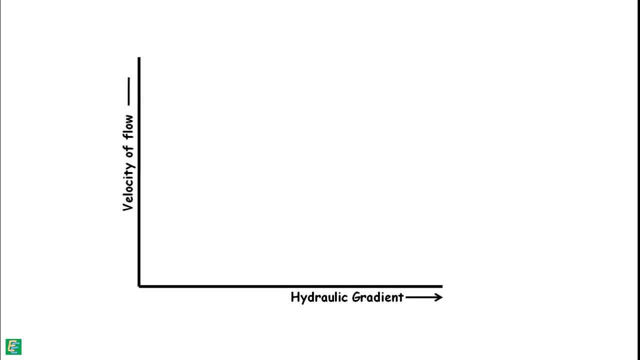 Here we hips the velocity of flow through the soil. If the double velocity of water is d会 mechanisms applied and velocity of flow, We will notice with the increase in the hydraulic gradient, velocity of flow also increases. We can divide this graph into 3 regions, namely zone 1, zone 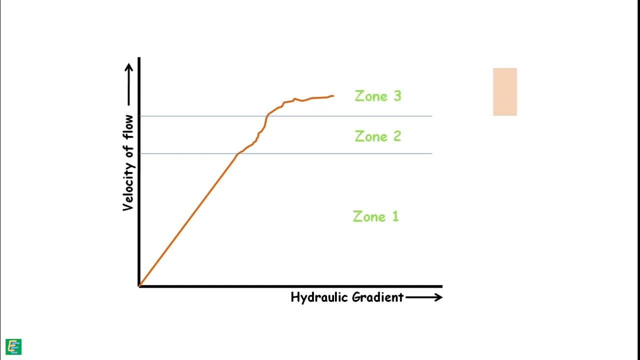 2 and zone 3.. Zone 3, where the curve is irregular, displays the turbulent flow of water inside the voids. Zone 1 depicts the laminar flow and zone 2 is transition zone. In laminar flow, the particles of water follow a defined path, such that the path of one particle never 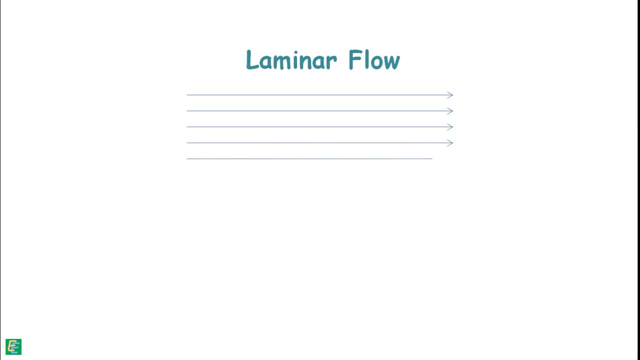 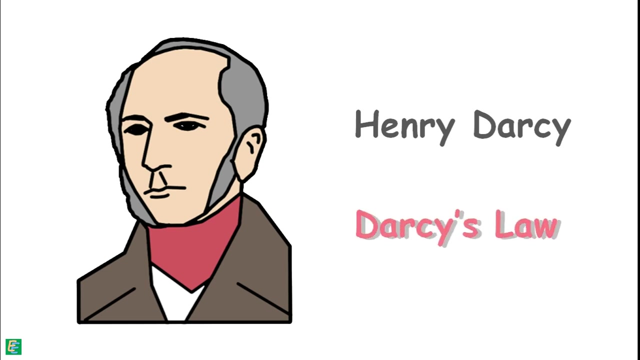 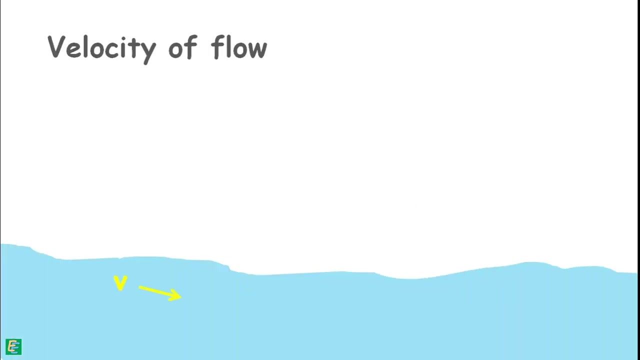 intersects the path of any other particle, While turbulent flow is irregular. We can observe in zone 1 hydraulic gradient and velocity of flow share a linear relationship. As an objective, we would like to know which is the coefficient of permeability of water velocity equation. 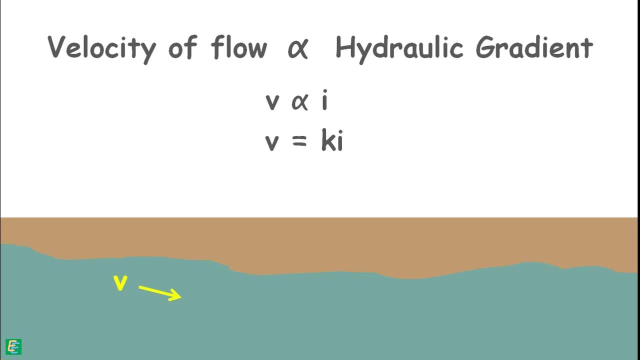 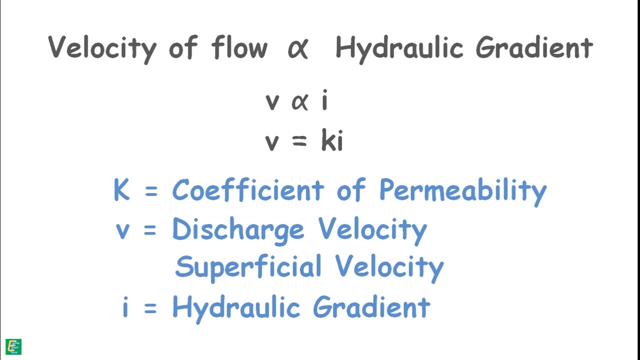 We can write it as this: by adding a proportionality constant, K. K is coefficient of permeability. V is the velocity of flow, which is also known as discharge velocity or superficial velocity. I is the hydraulic gradient. From this we can write coefficient of permeability as this: 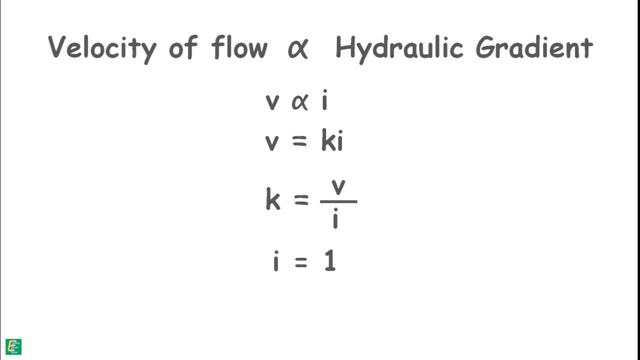 Here: if the hydraulic gradient is unity, that is, 1,, the coefficient of permeability will be equal to the velocity of flow. In other words, the coefficient of permeability is the velocity of flow of liquid inside the soil. if the hydraulic gradient is unity, 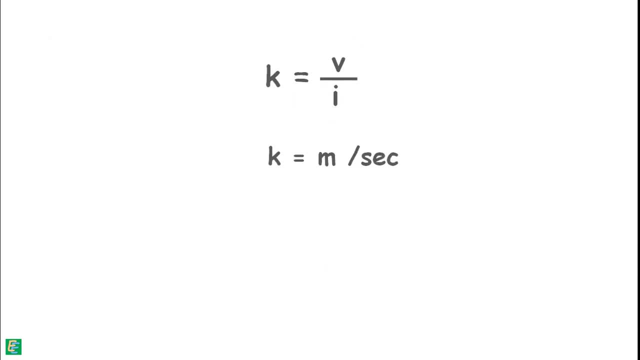 The coefficient of permeability has the dimensions of velocity. as hydraulic gradient is dimensionless because it is length divided by length, Discharge through the soil can be written as cross sectional area of the soil multiplied by velocity of flow. We can write the velocity of flow as this: 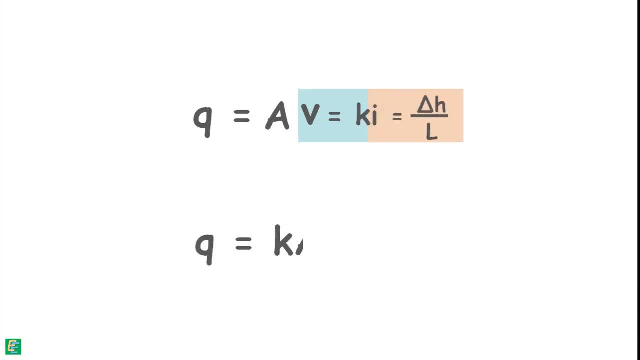 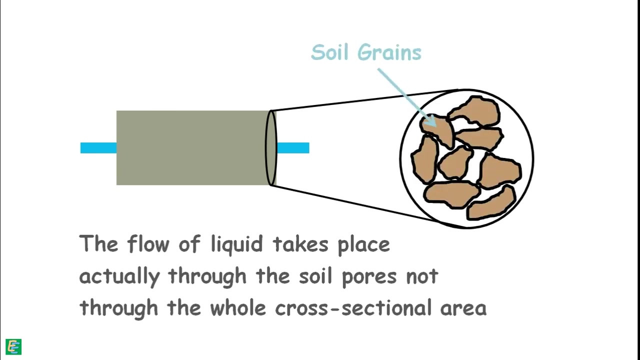 And also the hydraulic gradient can be written as. So equation will become: The flow of liquid takes place actually through the soil pores, not through the whole cross sectional area, Because primarily this cross sectional area is composed of soil solids and very less area is available for the voids. 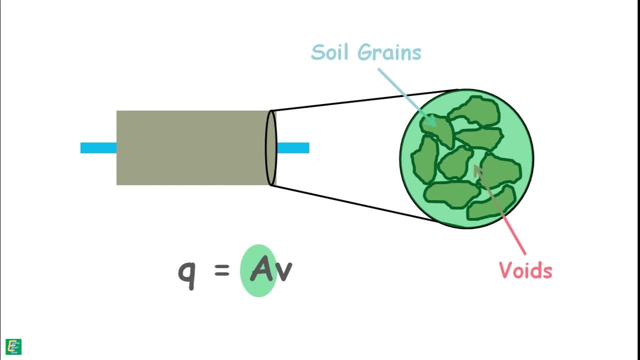 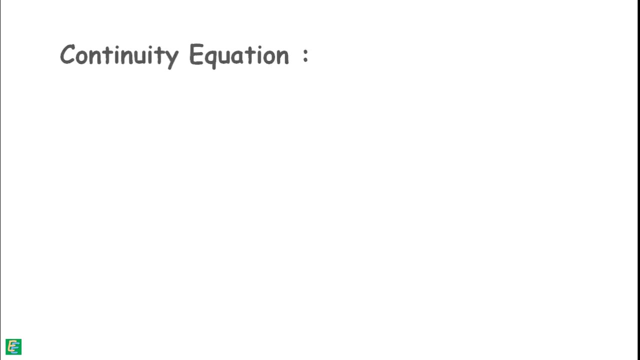 But for the calculations we have considered the whole soil area. So let's say average area of the voids is As, and the flow of water in the soil pores as velocity Vs. Using the continuity equation we can write: discharge through whole cross sectional area is actually equal to the discharge through its voids. 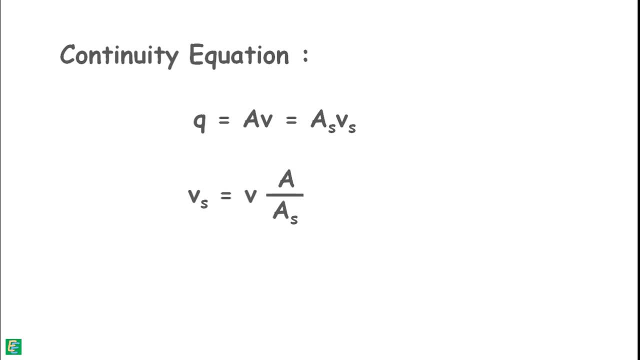 We can rewrite it for pore velocity. Now let's apply some mathematics and powerful brainy techniques and multiply both numerator and denominator by the length of specimen L. This is the total volume of soil sample and this is the total volume of voids. And if we write it as this, then we can see: this ratio is the porosity of the soil.